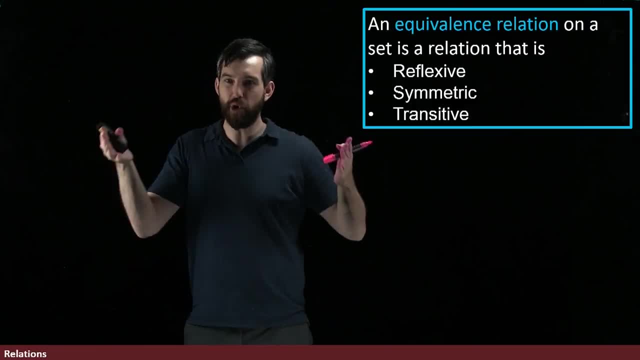 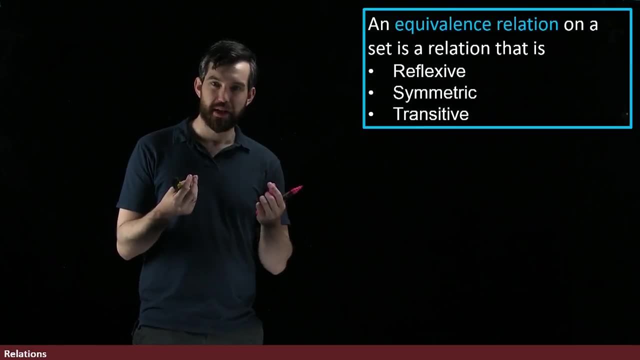 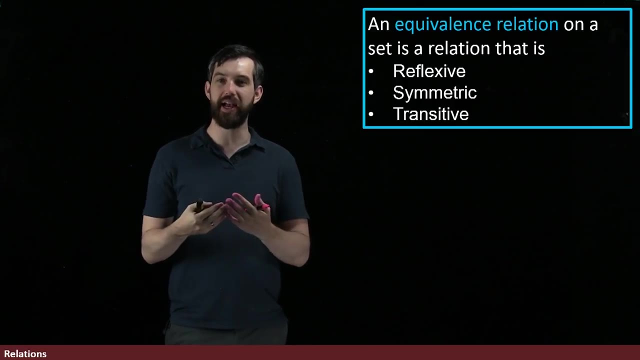 then the original three is equal to the third three. So equality is our notion of an equivalence relation, And indeed this isn't by coincidence. An equivalence relation is really trying to capture the essence of what equality should be, but in a slightly more. 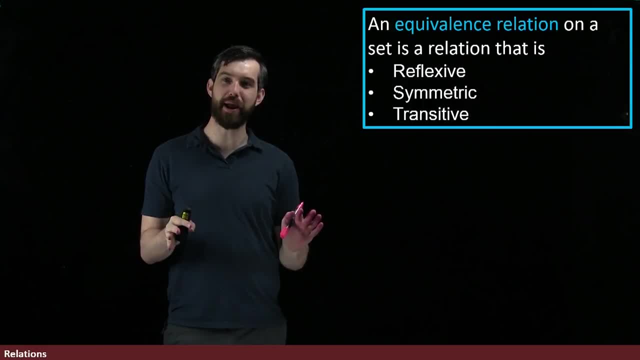 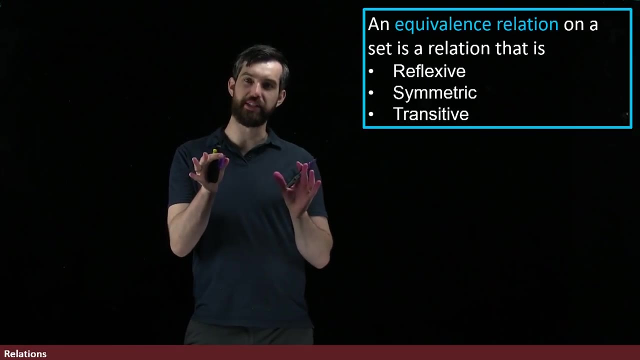 generalized concept. So this is going to become apparent in the second example of an equivalence relation that you've already seen before. You just didn't know to call it an equivalence relation, And this is equality of modular arithmetic. The second example I want you to consider is: 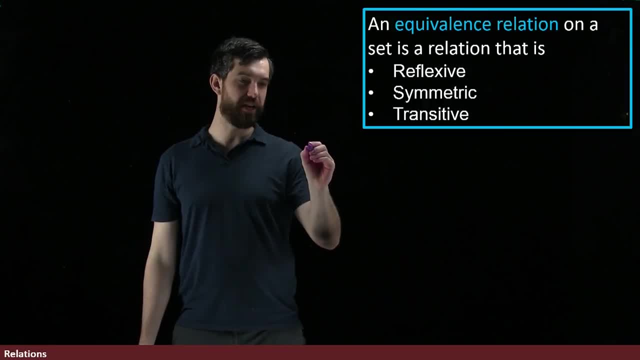 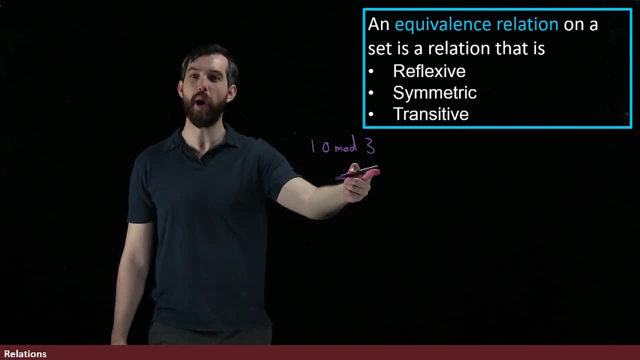 modular arithmetic. Suppose I have some expression like: how about 10 mod 3?? And we know that 10 mod 3 is going to be the equivalent of 10 mod 3.. And so I'm going to call it 10 mod 3.. And I'm going to 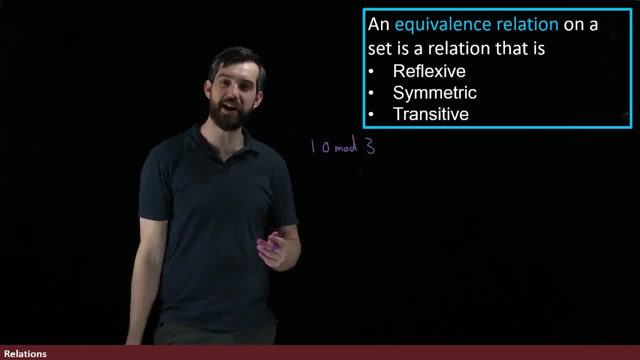 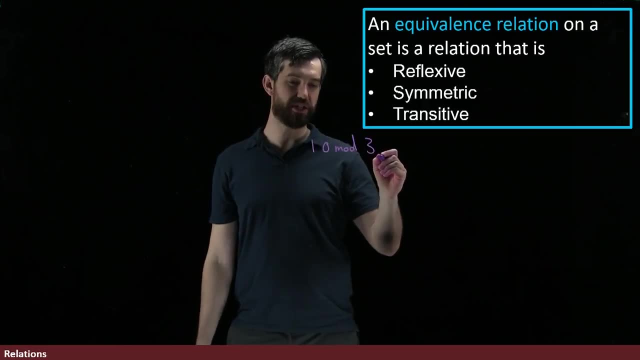 be the value of 1.. This is the remainder. If you take 10 divided by 3, or in other words you can say 10 is equal to three copies of 3 plus 1.. So we know that this is just going to be equal to the. 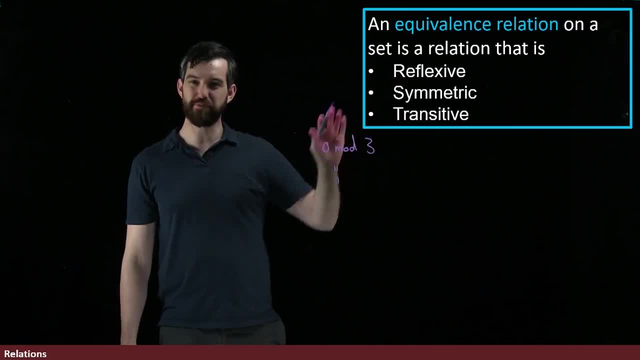 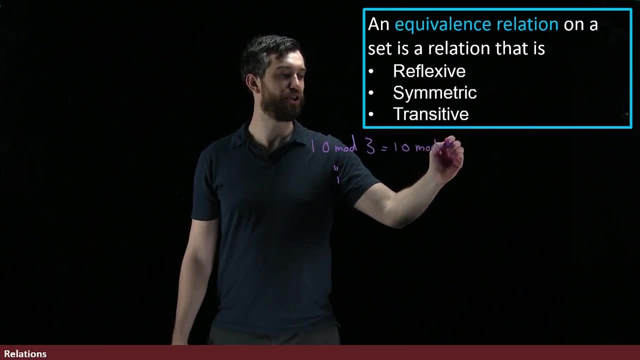 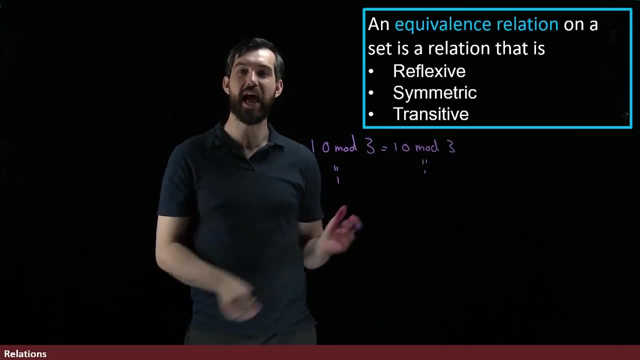 value of 1.. Doing the reflexive point is pretty trivial here. We're just going to be saying that this is exactly the same thing as 10 modulo 3, which is also equal to 1.. Of course it is So. indeed, it's reflective. The x is related to the x. 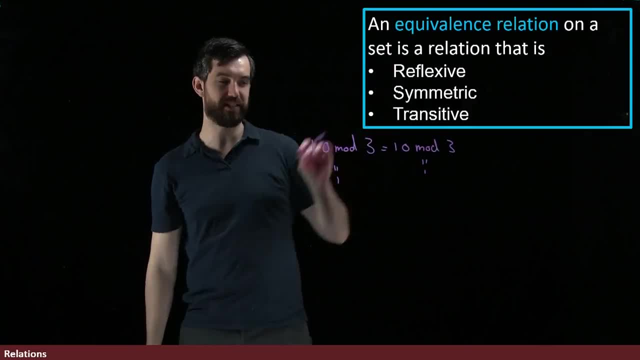 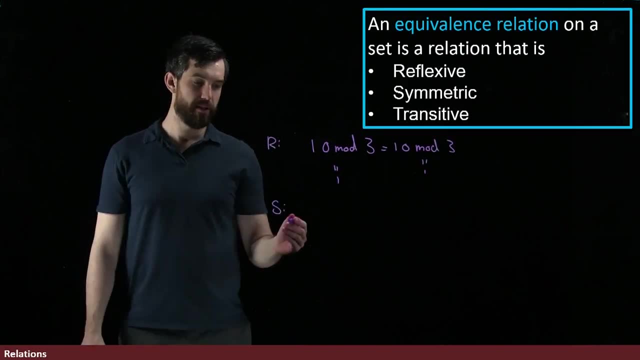 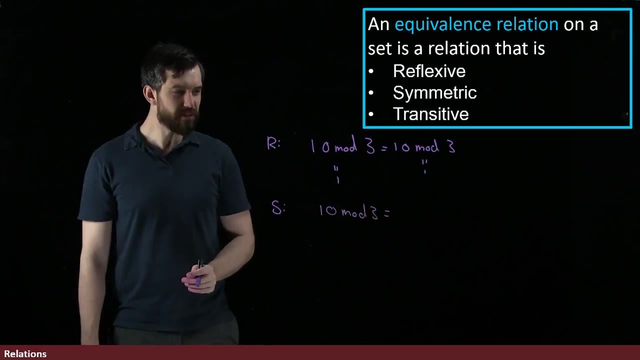 So equality in modular arithmetic obeys the reflexivity property. Well, that's a little bit less interesting. Now let's go and look at the symmetric property. If I look at 10 modulo 3, well, I can also say: I know this number is 1, but there's other numbers that are equal to 1 as well. 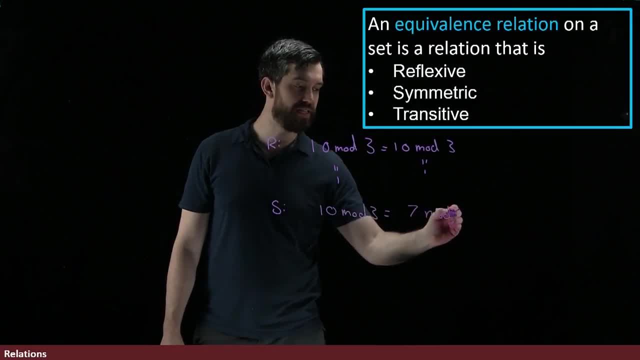 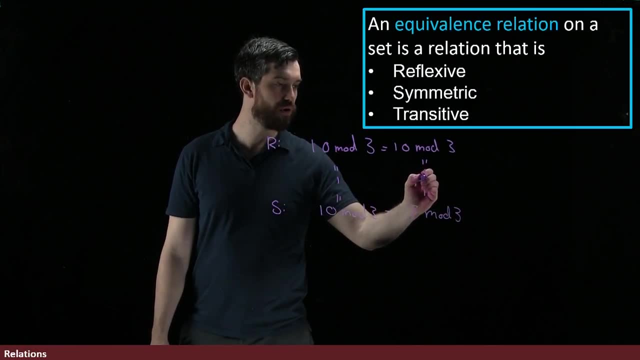 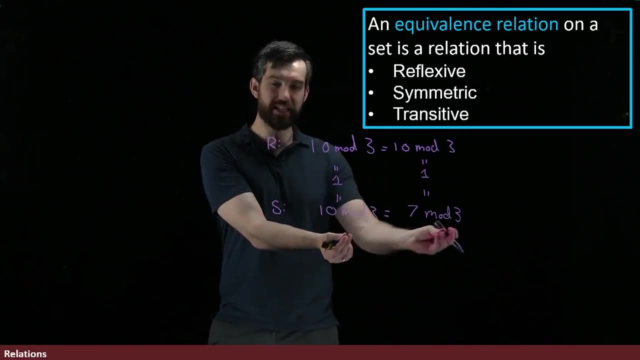 How about 7 modulo 3?? Indeed, 7 is twice 3 plus 1.. So it has the remainder of 1 either way. So all of these numbers just play out to be equal to these values just of 1.. But what we're saying is that in this 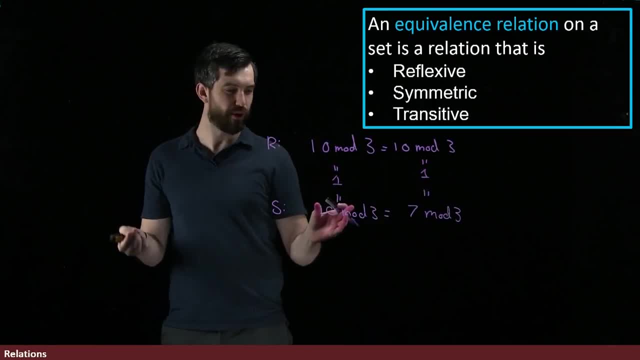 case we've got x is related to y, but notice that the x and the y, they really look different. now, In modular arithmetic, this equality here is this equality between these weird symbols, And we know that they're just equal to these numbers, but they really are represented symbolically very